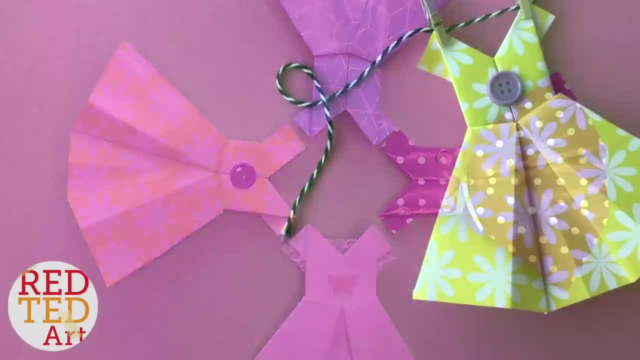 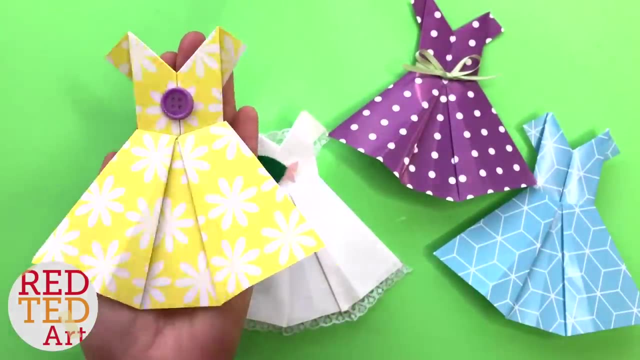 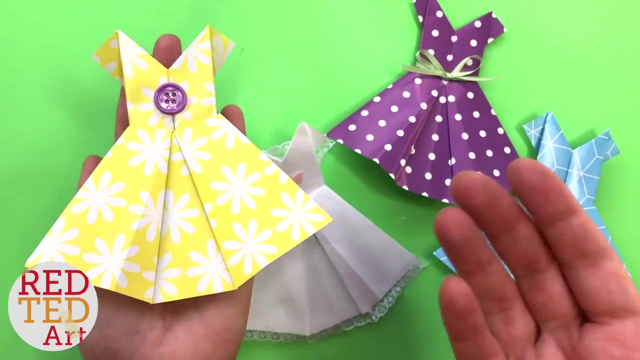 Hello, hello, Welcome back to Red Ted Art. Today, we're going to show you how to make these adorable origami dresses that you can then decorate in whatever way you wish. Now, this is probably one of the easiest origami dresses out there. It does have quite a few steps and if you're a beginner, 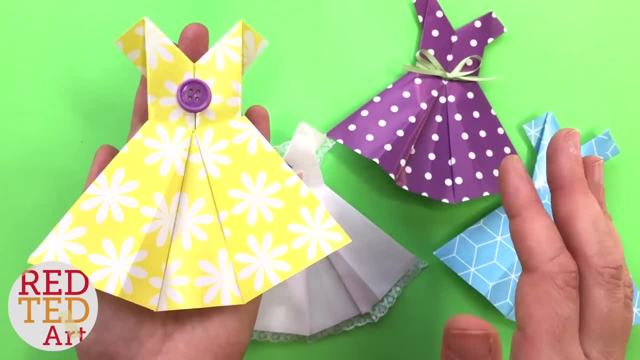 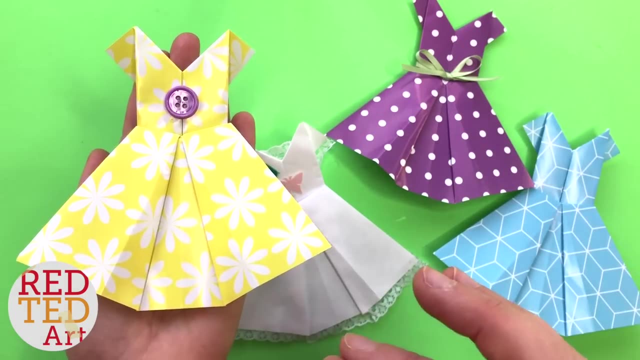 to origami. you might want to pause the video along the way, rewind and take another look, or maybe ask somebody else with a bit more experience to help you, But I do think the folds are quite easy. They're a good next project for people looking to learn the next skills. 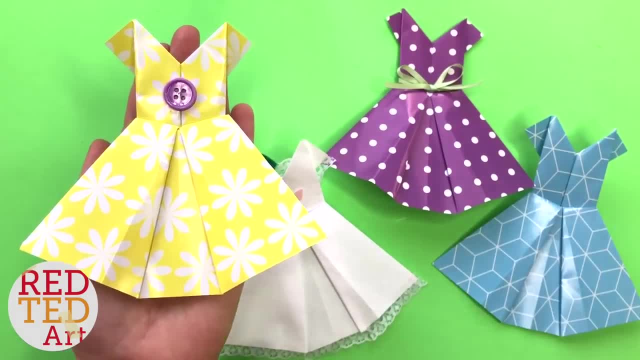 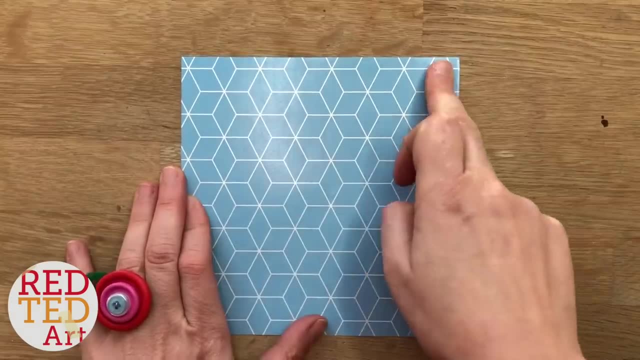 and I think the skirt, the little dresses, are so, so cute. So come on, let's take a look and see how they're made. So what you'll need is a square piece of paper. This is 15 by 15.. It really doesn't. 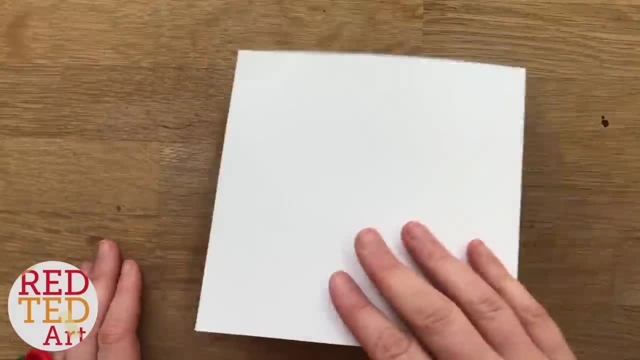 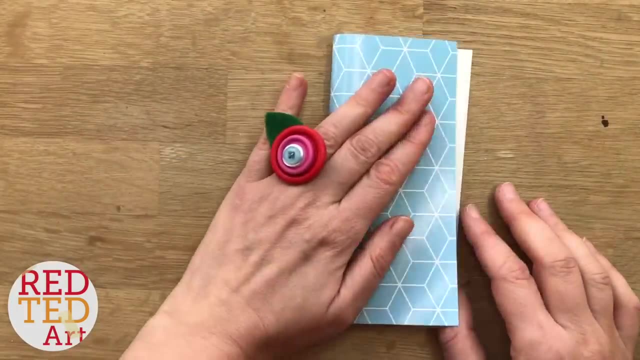 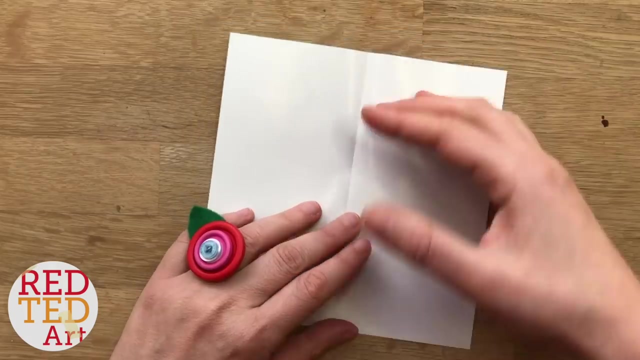 matter, it's just a question of preference. This is origami paper, so it's white and coloured on the other side, but you can use any paper you like. To begin with, you need to create some basic folds, So we're bringing one side over and lining it up with the other side. Open it and repeat. 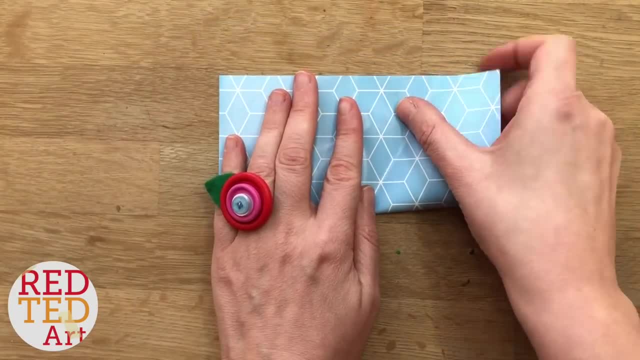 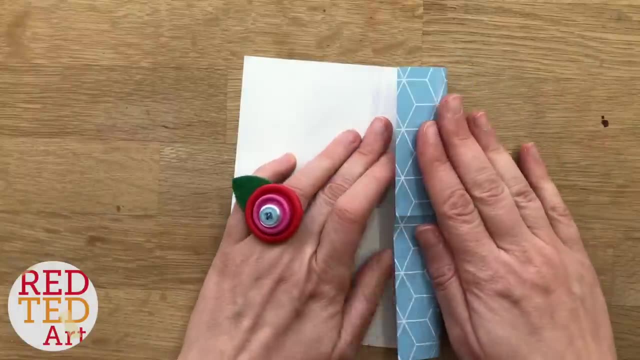 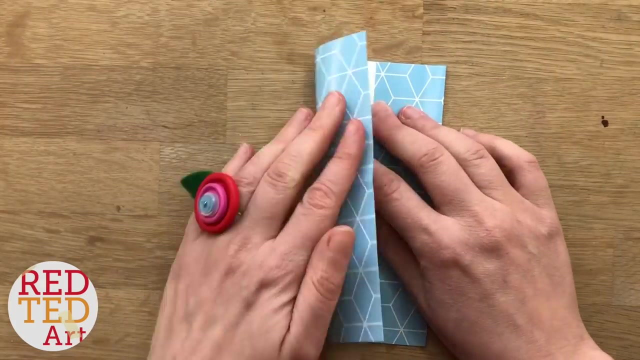 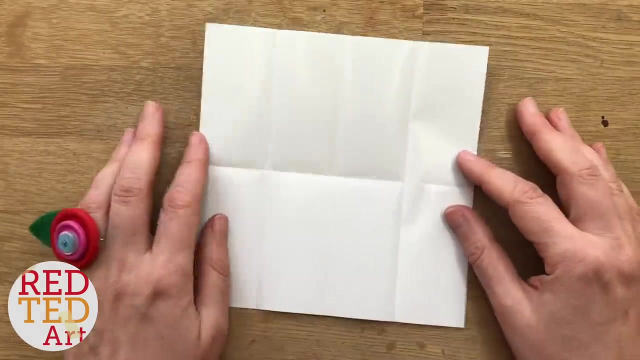 Open it. Now we're going to bring the sides in Again. we're just creating some basic lines up to the middle Hand. again, The neater you work, the easier. Open up, flip it round. Now you've got a line here in the middle. 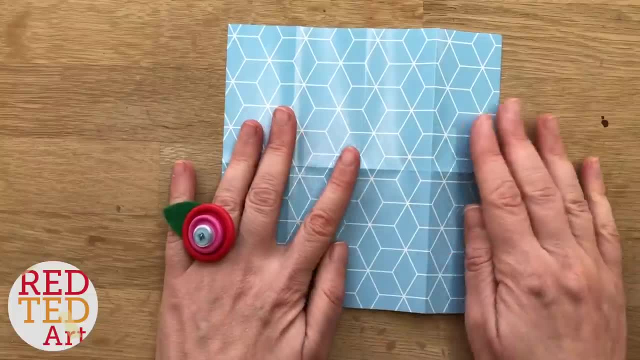 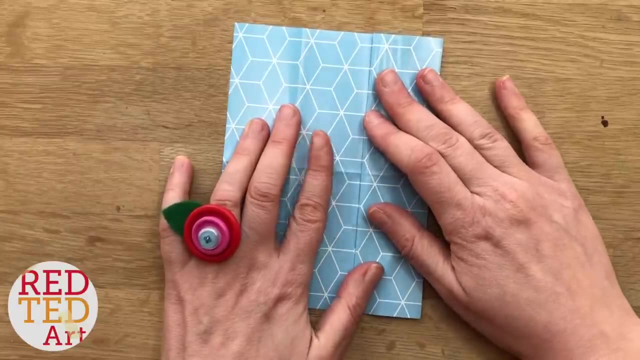 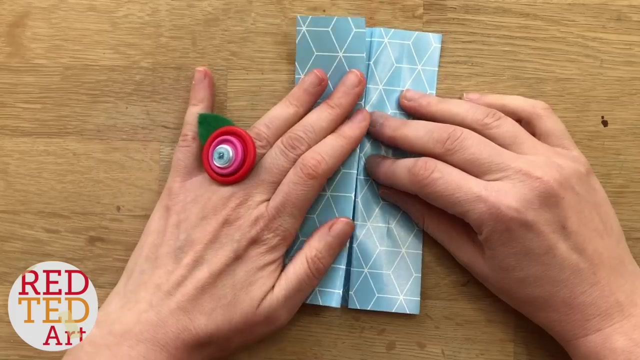 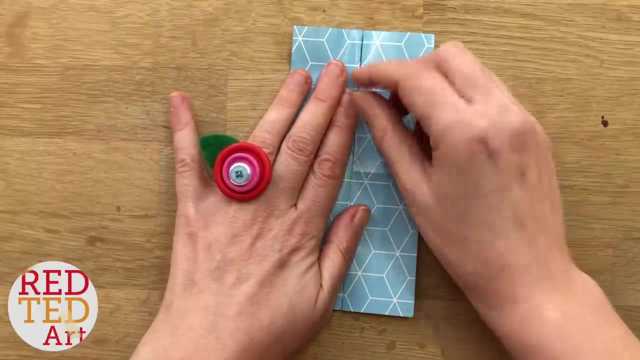 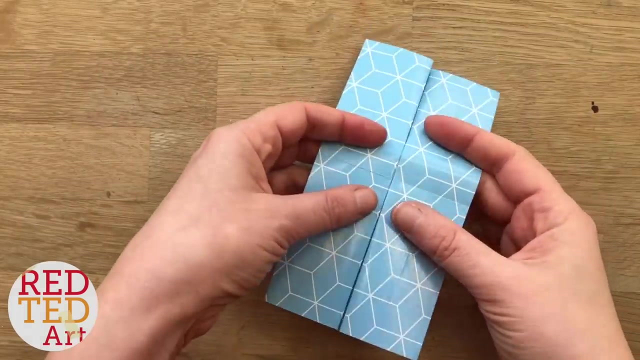 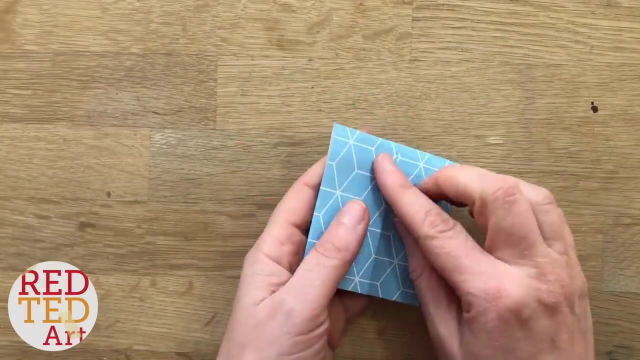 and a line here. You want to bring this line to meet and create a new fold. Again, you're bringing this fold and meeting it in the middle. You might have to push with your fingers to help get that in place. Now we're going to fold it in half and about one centimetre fold the 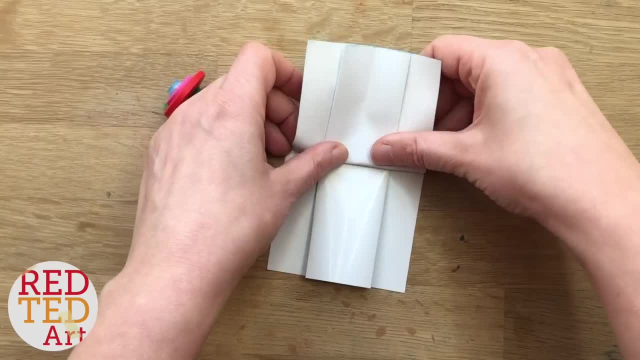 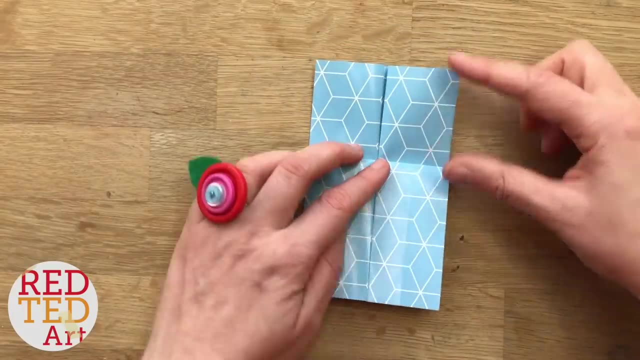 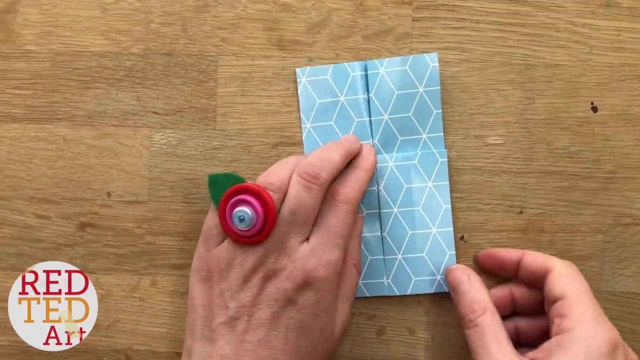 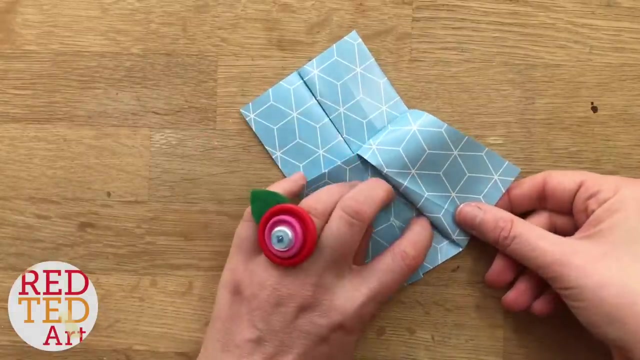 bottom up. Can you see? This is going to be your bodice, this is going to be your skirt. So make all your creases neat again. Now you give this a little tug, pull it out so that you come all the way out, and from the corner at the bottom, just crease it up. 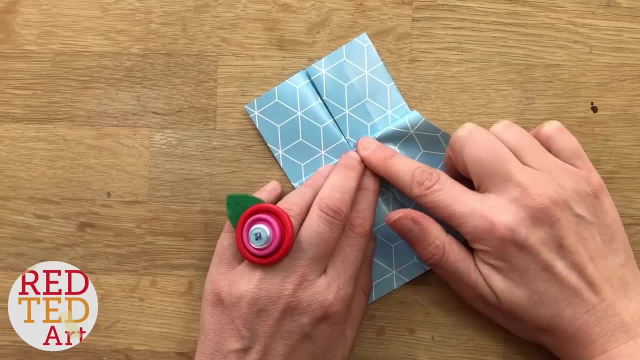 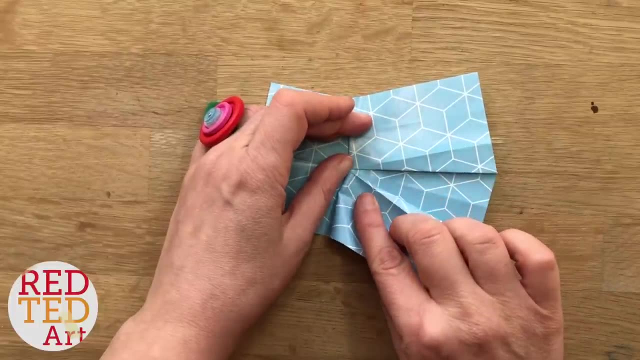 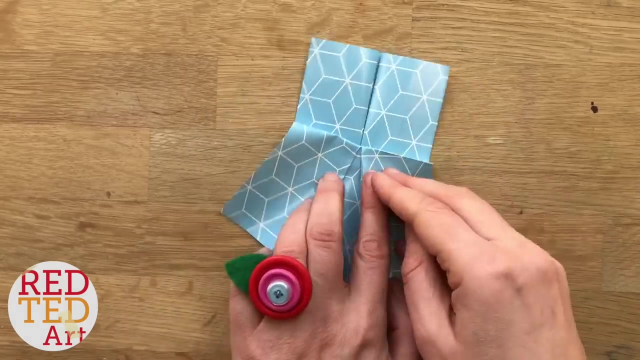 Once you've got that crease in place, you can crease up here Again on the other side. pull it out, so keeping that corner in place, pull it out till you get to the edge and give it a little crease and then repeat at the top. That's going to be your skirt, It looks. 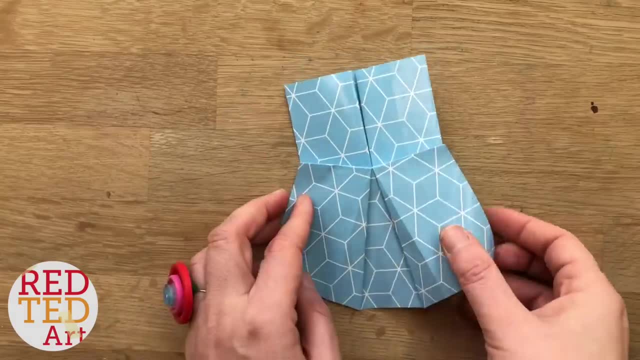 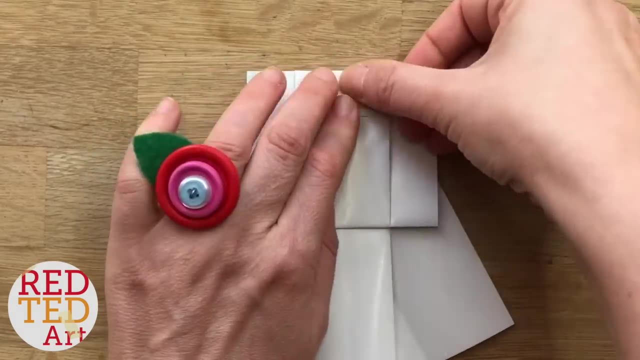 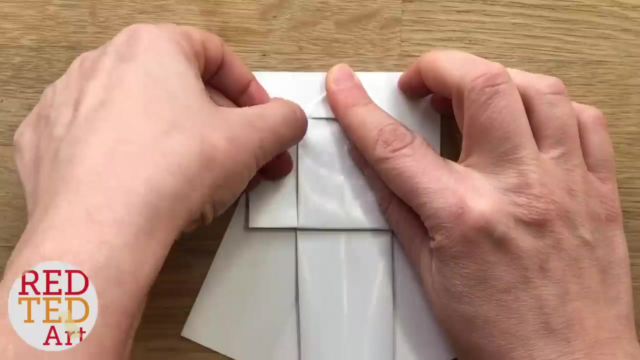 a bit big at the moment, but we'll add some folds in a minute. Flip it round, take this little corner and bring it in. Make a nice neat crease, especially here at the bottom. it's going to help And crease this in Again. make sure that corner is nicely creased. you're going 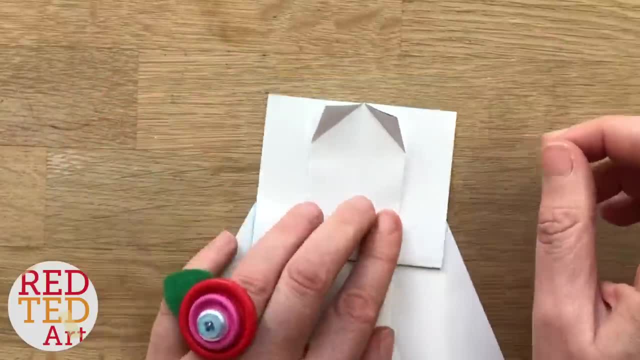 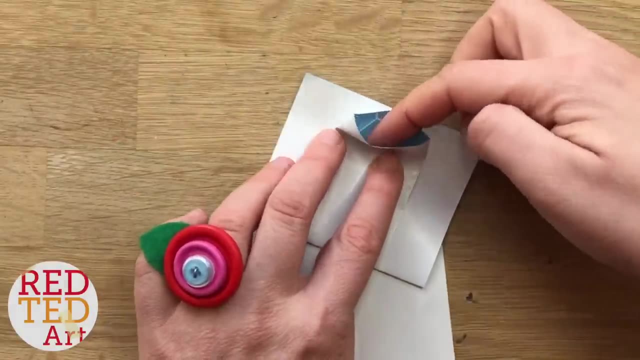 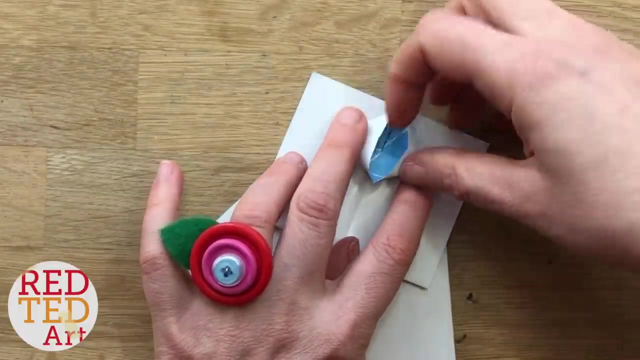 to need it in a minute. Open Now. this is probably the trickiest bit of the whole thing. Take one of the two flaps and fold down to that corner that we just created, And if you keep pushing, keep pushing, it'll fold down. 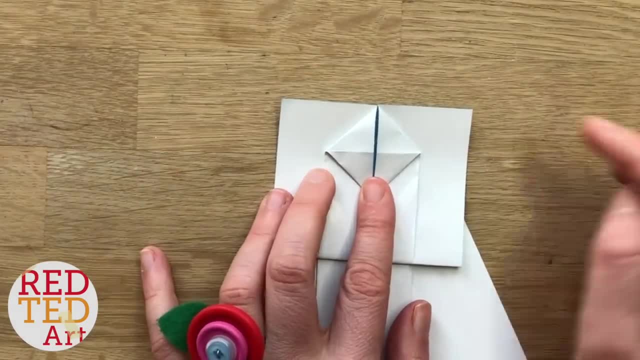 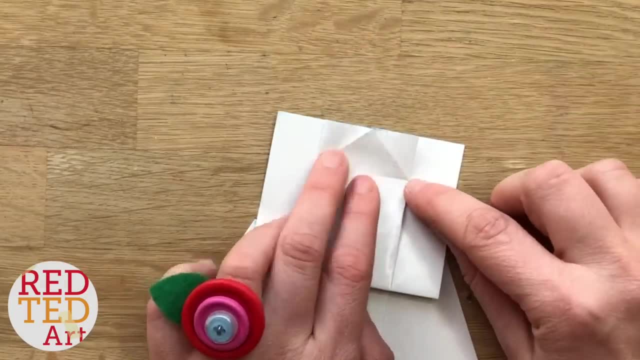 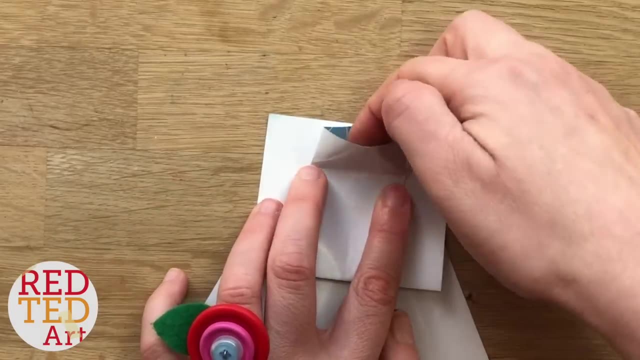 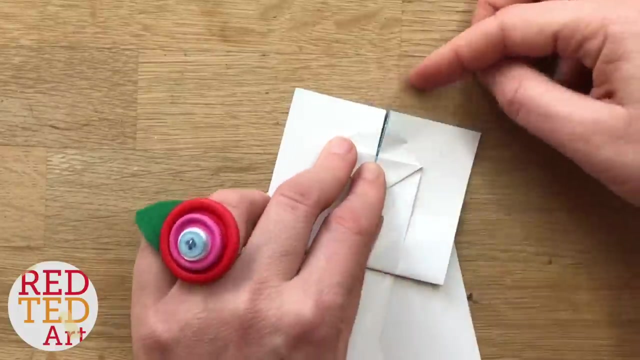 the hardest part. I can show you that again. When you've created these two corners, you've folded it, Make a nice, neat corner, Open it, Pull and down, Say, we're almost there, Now, take this, fold it in. This is going to create your little bodice top And fold this one and fold this. 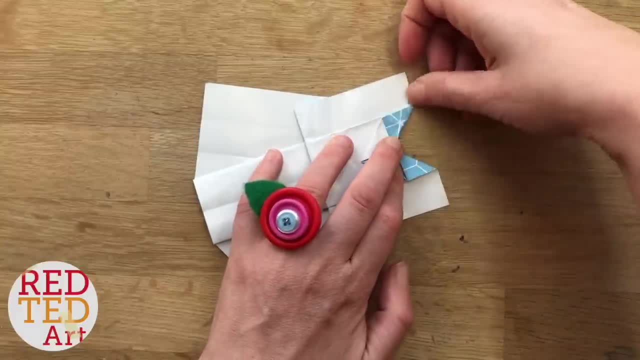 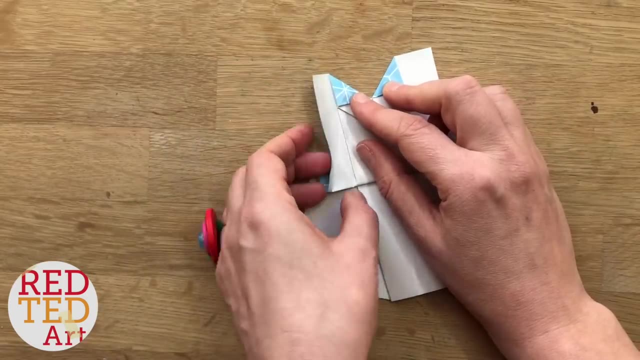 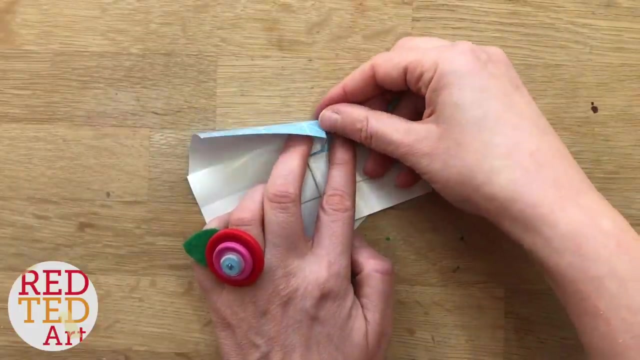 one Looks like this: Now, we're going to shape the arms. See that straight line here. We're going to fold that over, start at the top and, as that comes down, this is flapping over, isn't it So?